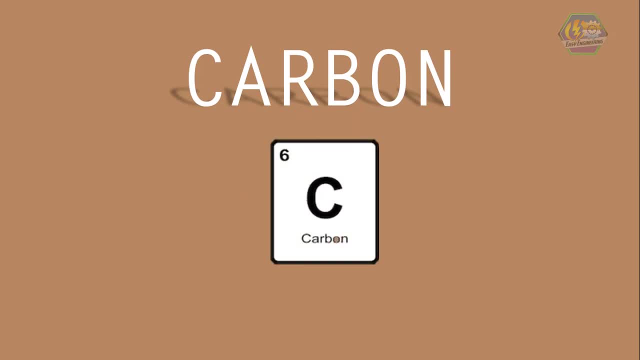 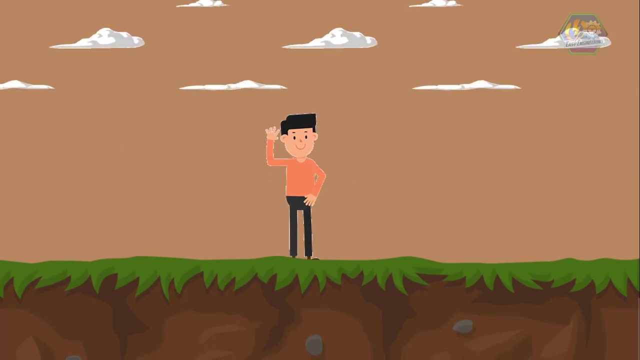 Carbon is one of the most important elements to the living things. All living organisms have carbon as the basis for life, because at some point we are all made of carbon. That's why we are sometimes called carbon-based life forms. Carbon is also found in some non-living things. Carbon is found in you, in the ground and even in the air. 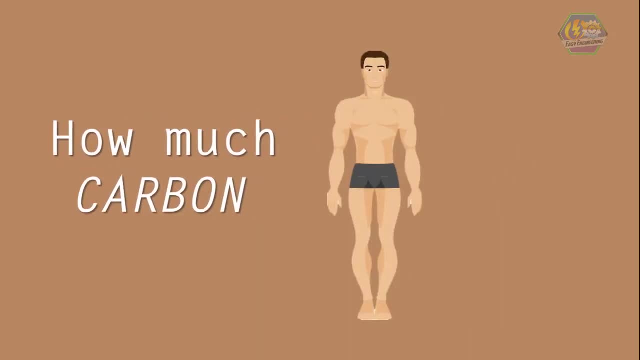 Fun fact learners. did you know how much carbon is in the human body? Well, it actually makes up about 18% of the human body. So if you weigh 100 kilos, then you have 18 kilos of carbon in you. 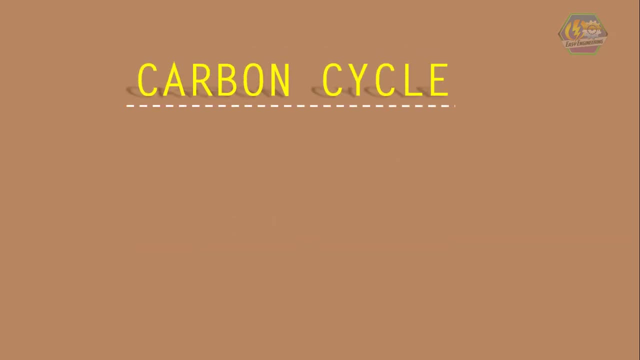 Since our topic is the carbon cycle, you might think it is using carbon and recycling it after. You're not wrong in that case. Now you might have heard of atoms, but don't believe them, because they make up everything. Mm-hmm, That was a joke. 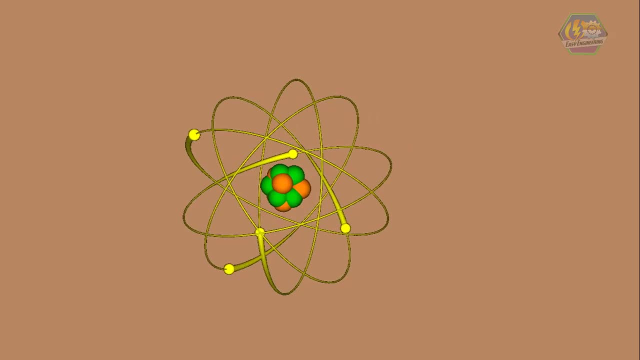 Well, in fact, they do make up literally everything. Everything in the world is made up of atoms. They are the smallest thing there is. Carbon atoms are one of them, and if you combine a lot of carbon atoms, they form carbon. 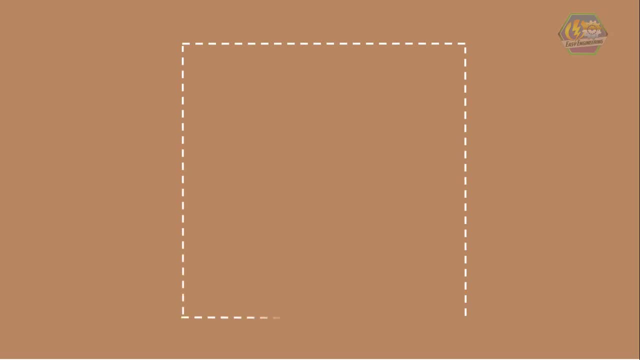 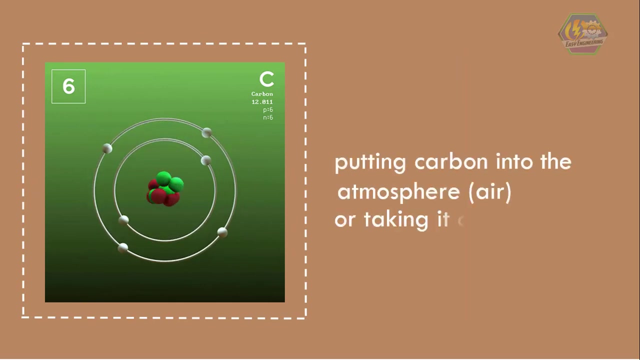 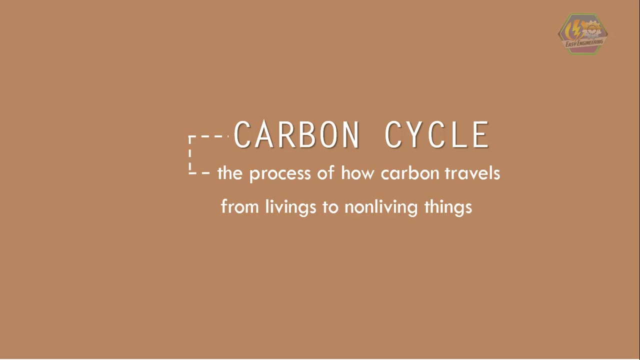 Some carbon atoms, although we cannot see them, are moving around non-stop. That's because carbon atoms are used by all sorts of processes on our planet, Processes like putting carbon into the atmosphere or taking it out. So, basically, the carbon cycle is the process of how carbon travels from living things to non-living things. 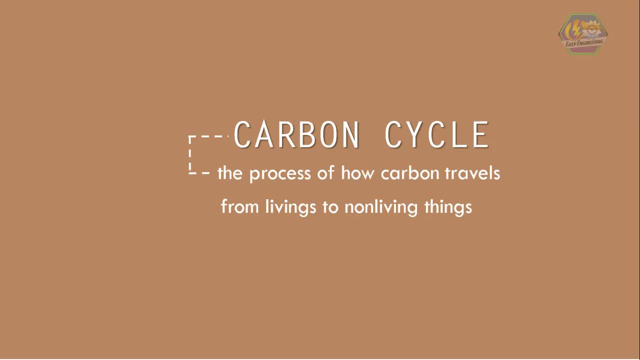 Now there's some ways how carbon travels around the world. Let's look at a basic example. Carbon dioxide is always present in the atmosphere. Part of it has some carbon in it and the other part is oxygen. Plants use carbon dioxide from the air to make food. 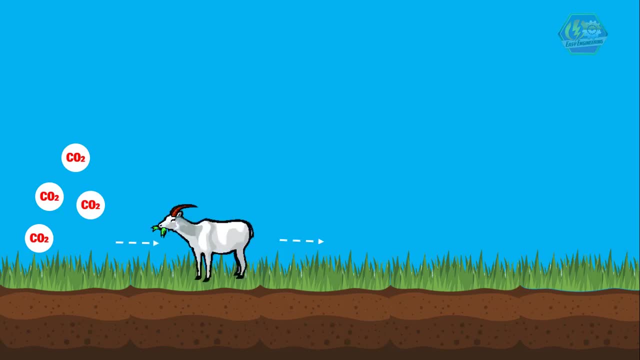 Then some animals eat those plants that have carbon in it. Sometimes we eat the animals and then we fart. That fart is also a form of carbon dioxide. So there we go. The carbon was returned to the atmosphere. A simple carbon cycle. 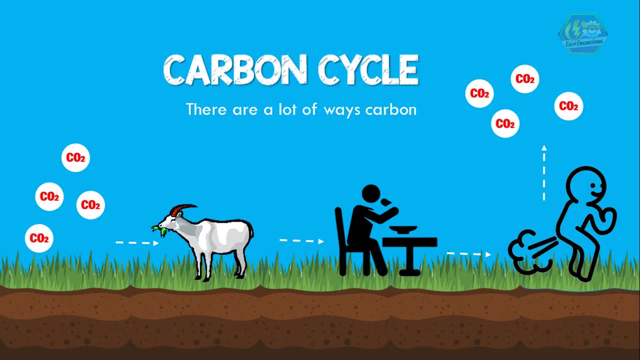 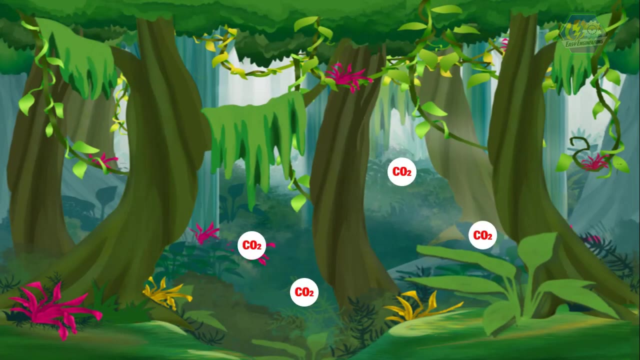 But there are actually a lot of ways carbon is reused by the environment. So let's take a deeper look. Let's see first how carbon is taken out of the atmosphere. Nature always sucks the carbon out of the atmosphere. One example we know is the process called photosynthesis. 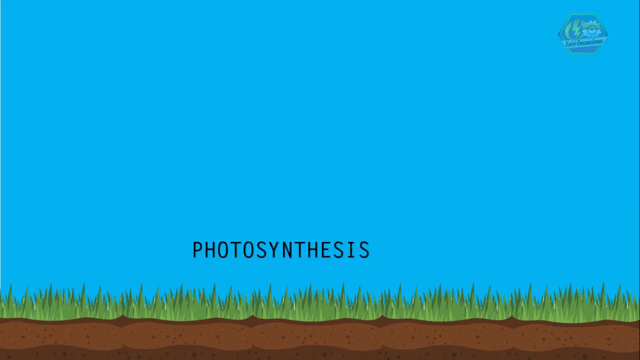 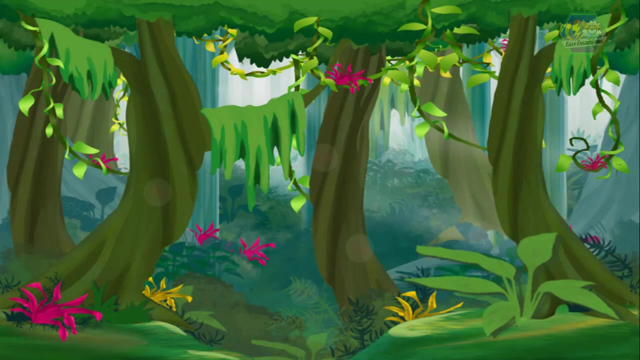 Plants use this photosynthesis or food making to produce energy and grow. They take carbon dioxide, sunlight, nutrients from the soil and water, then turns it all to oxygen and sugar. Most of the plants like in the rainforest actually help remove or clean the atmosphere of carbon dioxide. 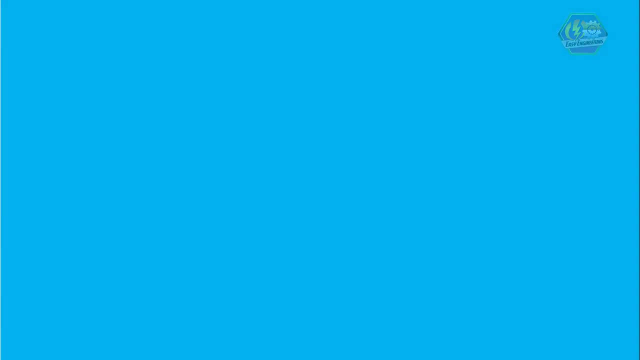 So keep planting more trees. Next is the ocean. You might want to ask: how does the ocean use carbon? Well, ocean water helps a lot in removing excess carbon from the atmosphere. Carbon dioxide in the air reacts with the seawater to make carbonic acid in the ocean. 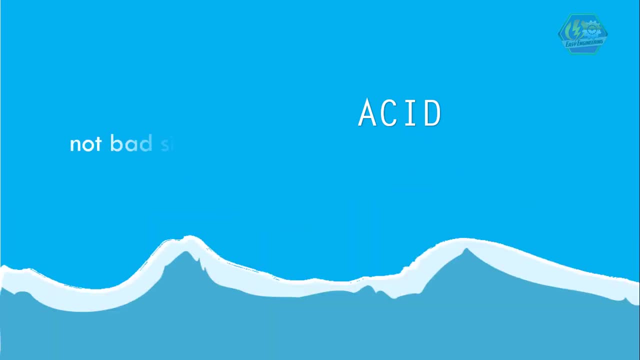 Acid. Is that bad? Well, not really, since there's only enough for the ocean, Although if there's too much carbonic acid it can cause acid rain That can destroy plants. But mostly carbon dioxide in the ocean is good, since the carbon combines with calcium to form calcium carbonate. 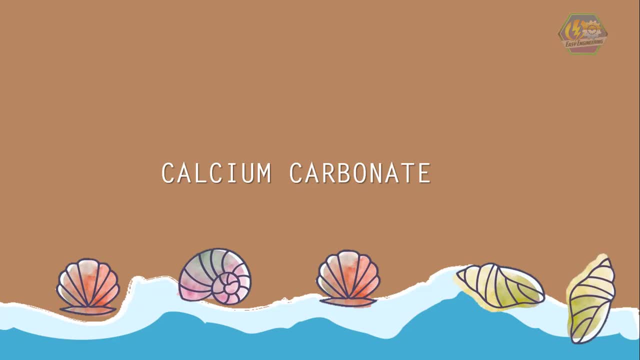 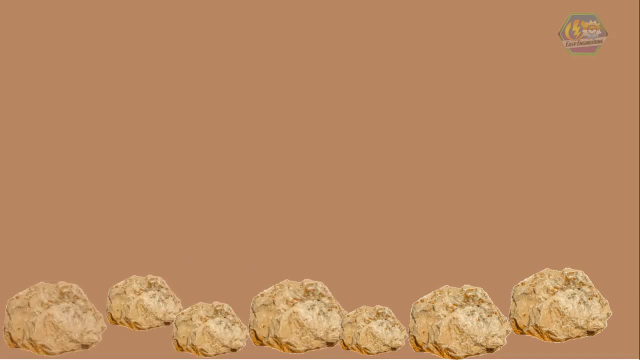 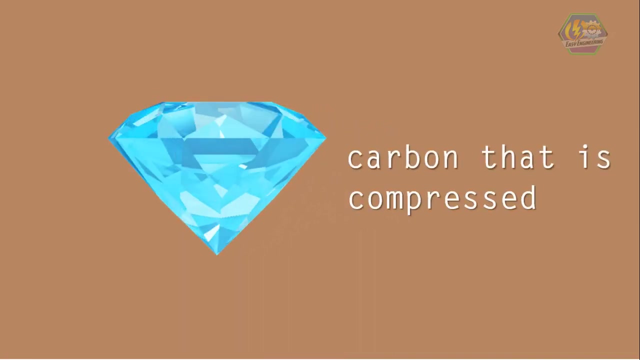 It is the main component of sea shells. A lot of sea animals use shells and eventually it will become sedimentary rock like limestone that helps keep the surface together. Fun fact learners: did you know that diamonds are just carbon that is compressed? 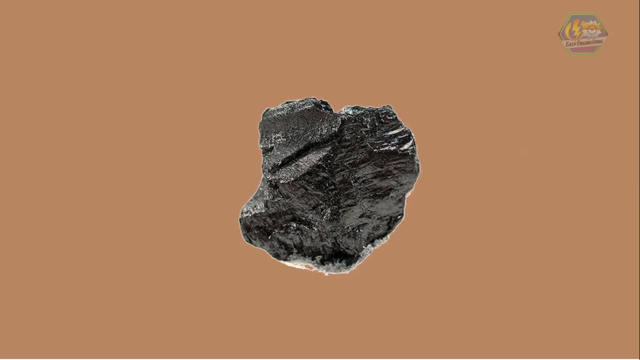 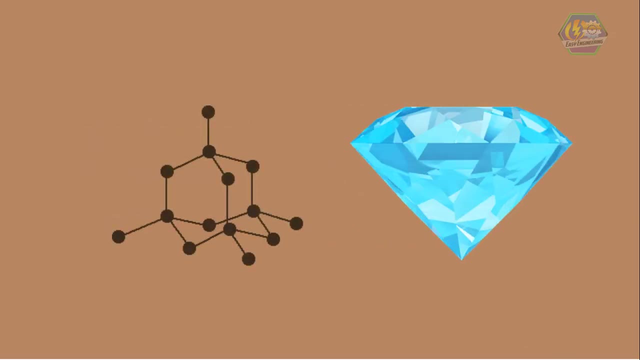 But when we imagine carbon it's pitch black, right. Well, diamond is actually a solid form of the element carbon, with its atoms arranged in a crystal structure. That means with proper spacing and arrangement of carbon you can form diamonds. 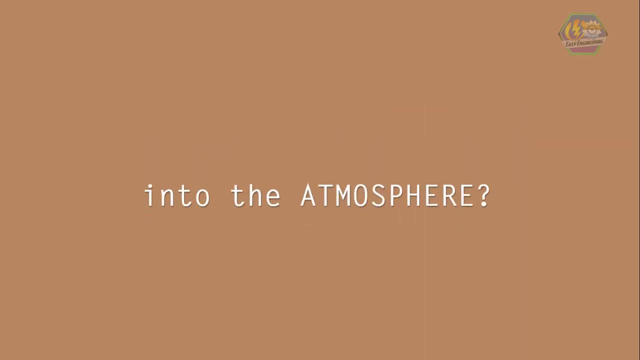 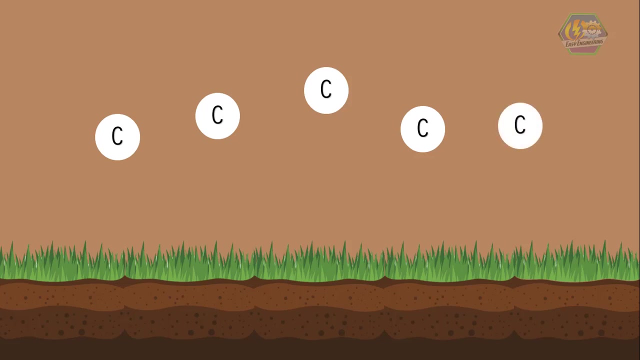 Now, how about moving carbon into the atmosphere? There's also some processes, not just one, of how nature adds carbon to the air. These processes are called sources. One example is respiration, or breathing. Every time we breathe, we inhale oxygen and in return, we exhale carbon dioxide.